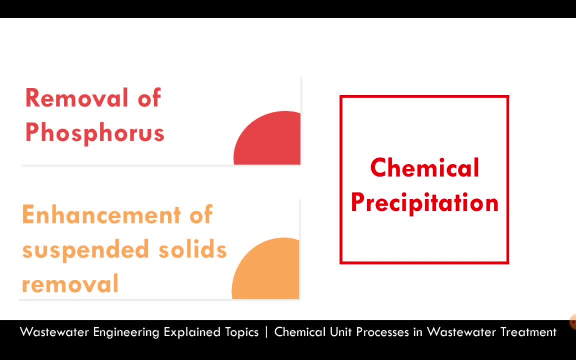 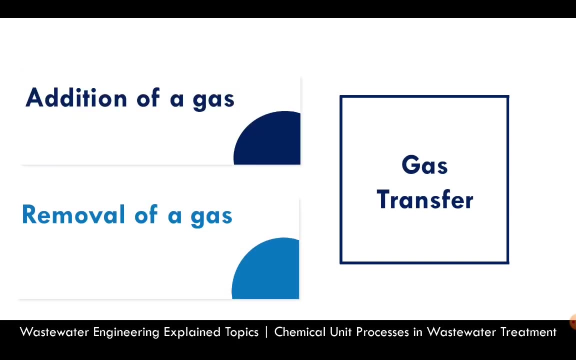 ion chemical that creates settleable solids. okay, phosphorus is the example that is removed by addition of calcium, iron and aluminum salts. all right then. the second chemical unit process is chemical precipitation. the second chemical unit process is gas transfer, in which both the things take plus: addition of a gas and removal of a gas. okay, now, in West water treatment we 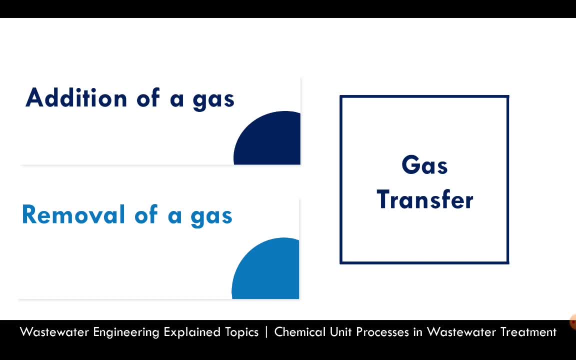 can add oxygen for improving the performance of biological units, then stripping or removal of toxic organic can be done, which is removal of a gas. okay. then we can change the percentage CO2 inside West water for the better pH control. then we can remove that. this is gas removal process of ammonia, which is there in gas transfer as the unit. 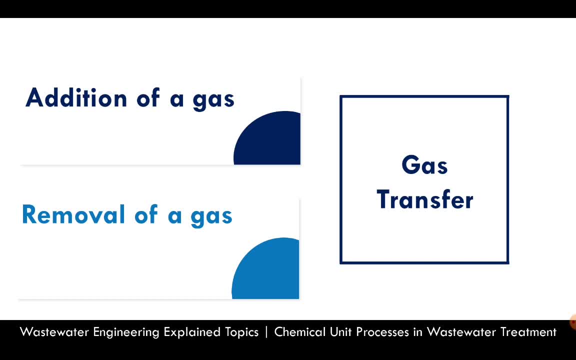 professors, then chlorination may be added in the West order for disinfection purposes, in format of gas, which comes under addition of gas. all right, then adsorption. adsorption is a surface phenomenon in which molecules, that is, adsorbate, adder to a surface, for example activated carbon, which is a common at. 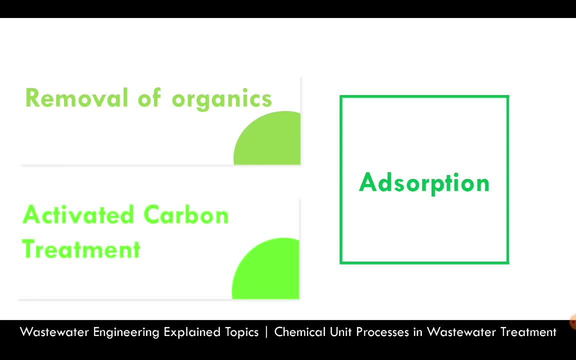 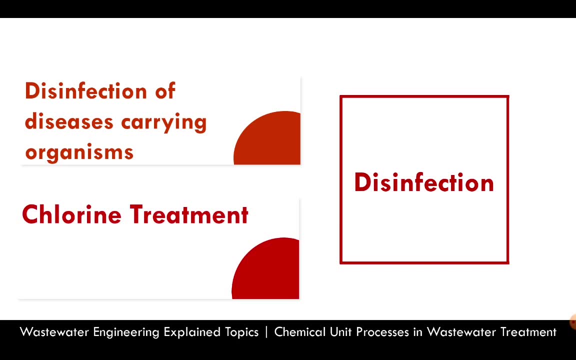 absorbent. also, heavy metal can also be removed by using the concept of absorption. all right, then the fourth unit process in chemical unit process is disinfection, which means killing or inactivating most of the microorganisms which are present in the west water. okay, chlorine treatment. 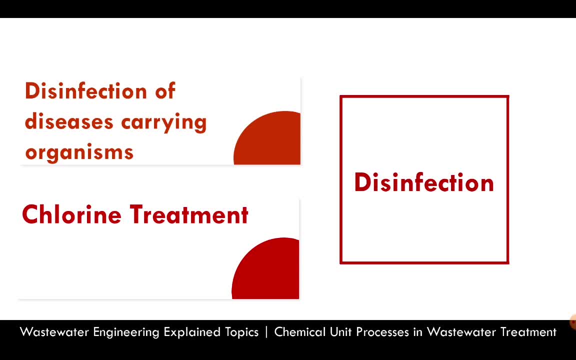 is the most common disinfection process in west water. okay, then dechlorination. okay, dechlorination means what removal of chlorine- free, combined or residual chlorine- is removed from west water using sulfur dioxide, sulfide salts such as sodium sulfide is there? sodium bisulfite is there? or? 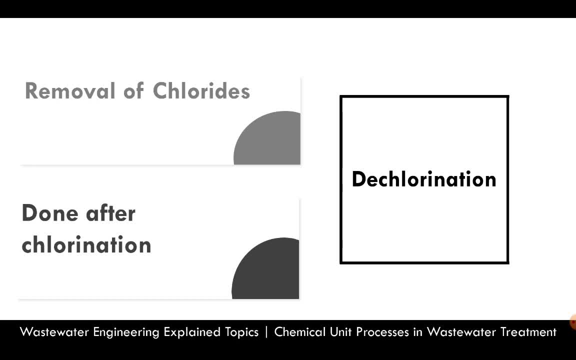 sodium metabisulfite is there. okay, mostly the dechlorination process is carried out after chlorination. dechlorination process is carried out after. chlorination process is carried out after to take care of the residual or extra chlorine which is present in the west water. okay, so these